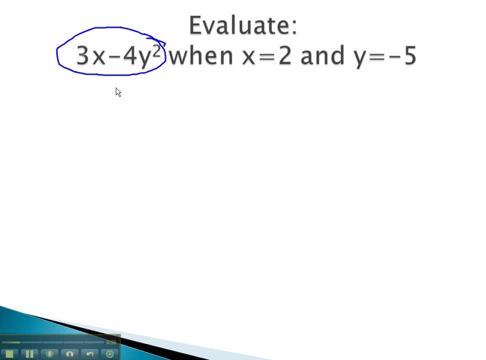 3x minus 4y squared, There's two variables, the x and the y, which are representing unknown numbers. Well, this problem wants us to evaluate when they tell us the x is representing the number 2, and the y is representing the number 5.. 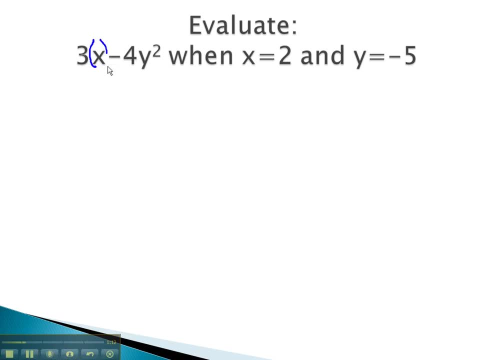 What we can do is we will replace the x and the y with parentheses around the number it represents. So this means we have 3x. x represents the number 2.. Minus 4y, y represents the number negative 5 squared. 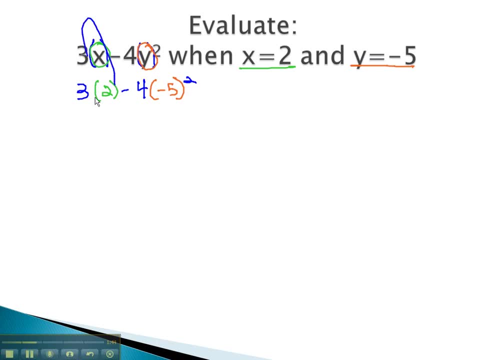 And all we've done here is we've replaced the x with 2, and the y with negative 5, and now we have an order of operations problem which we can solve. Order of operations is going to ask us to evaluate the exponent first. 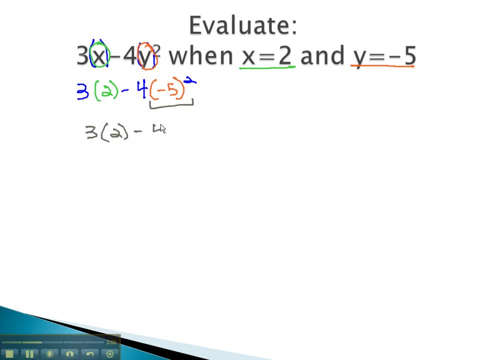 So we have 3 times 2, minus 4, times negative, 5 squared is positive 25.. Next we multiply from left to right. 3 times 2 is 6, minus 4, times 25.. Continuing to multiply from left to right. 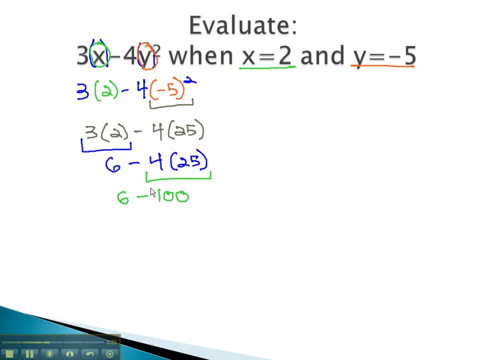 we get 6 minus 100.. And finally, when we add the opposite 6 and negative 100,, the negative 100, 5 is bigger, and when we subtract we get 94, or negative 94 for our solution. 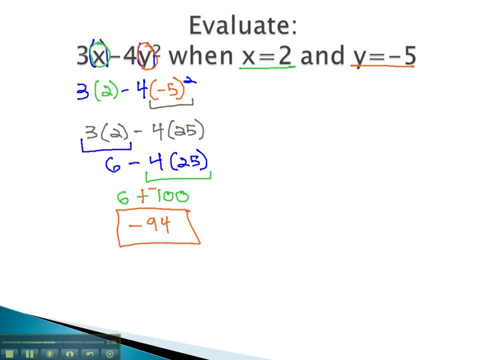 So we can evaluate an algebraic expression by replacing the variable with the number it represents. Let's try one more example. Here we have a c squared over 3a plus 4b. We can replace the c with what it represents: 6,. 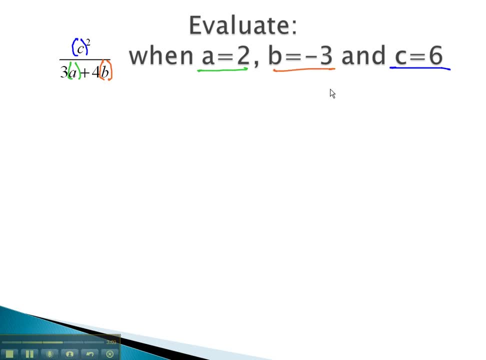 the a with what it represents 2, and the b with what it represents negative 3.. When we do that, the c is now a 6 squared over 3a, which is now a 2, plus 4b, which is now a negative 3,.